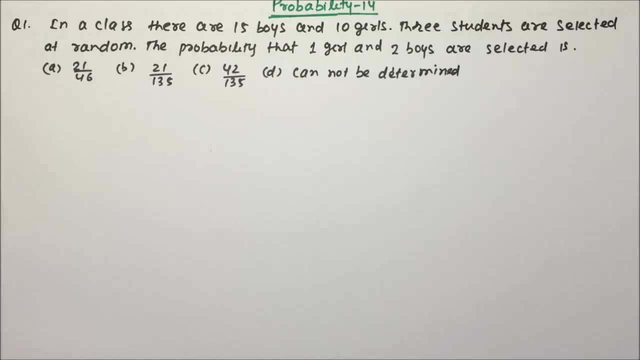 will be asked, And our today's questions are very important and this kind of questions will be mostly asked in your exam. So I will suggest you please watch the previous videos and probability so that you understand the concept and then you can solve the questions. 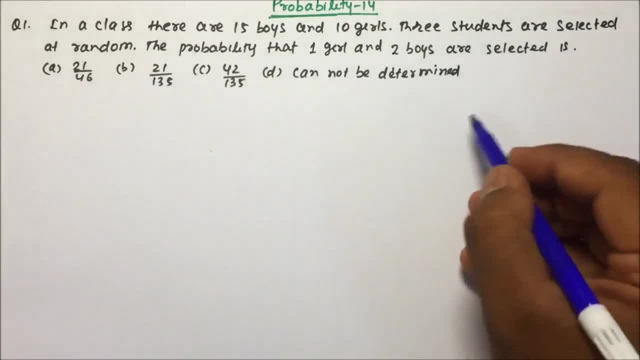 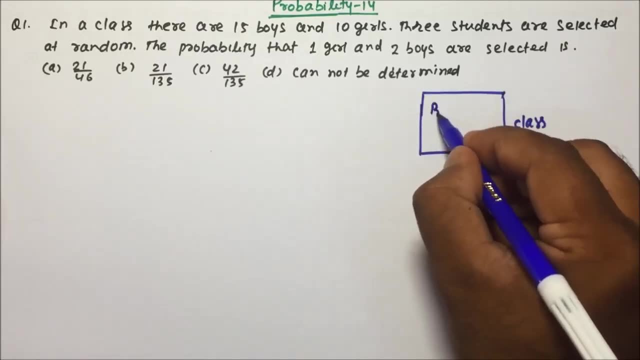 easily. So let us start with the question number 1.. So in a class there are 15 boys and 10 girls are there. So suppose there is a class, is there? This is my class, In that number of boys is 15 and the number of girls are 10.. So if we will talk about 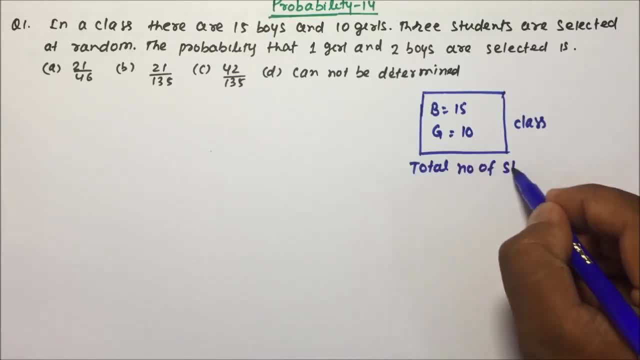 the total number of students. So total number of students will be equal to boys plus girls, which is nothing but 15, plus 10, which is nothing but 25.. So there are total 25 boys and 10 girls. Students are there in the class Now. 3 students are selected at random. So, friends, 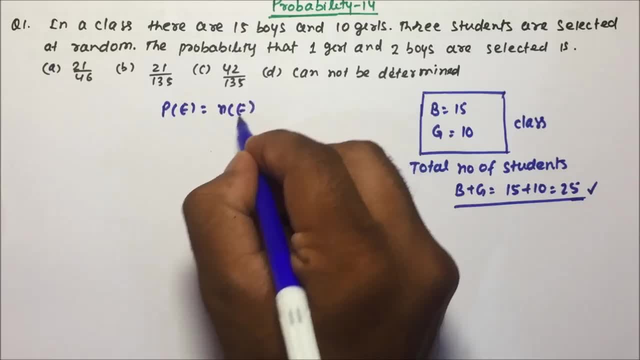 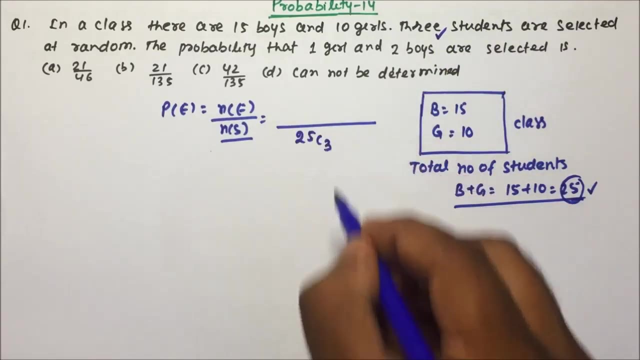 basically we have to calculate probability. So probability will be always equals to NE by NS. Now, so if we will talk about the NS, then what will be NS? So NS will be nothing, but so total 25 students are there and 3 students are selected at random. So 25 C, 3, 25 out. 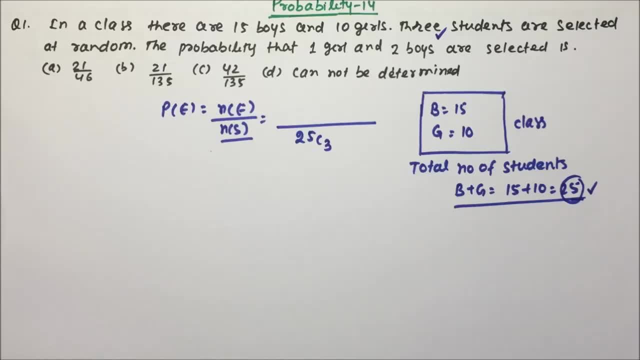 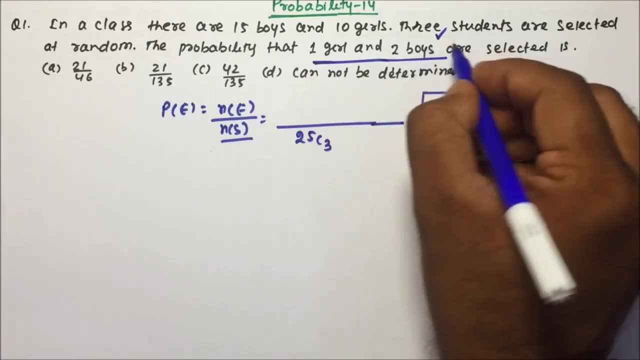 of 25,. you are selecting 3. So we will use combination C. is the selection Now NE in your favor? So what you want? The probability that 1 girl and 2 boy are selected Now if AND is there, if OR is there. 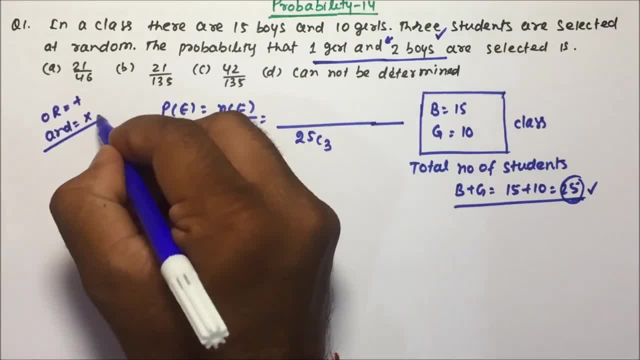 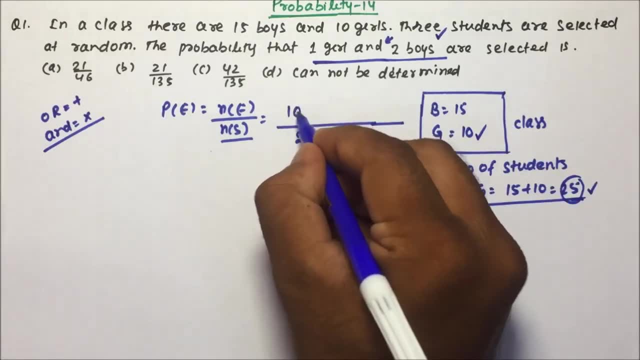 means we have to add, and if AND is there, we have to multiply. Right, friends? Okay, the probability that you want 1 girl and 2 boys. So if you want girl, then select from the girls. So 10, C, 1, AND, AND means multiplication. You want 2 boys, then you select from the. 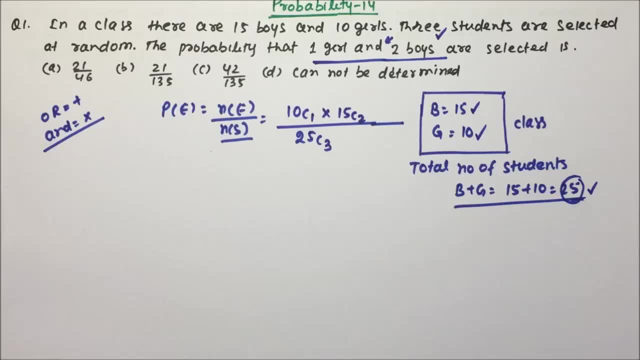 boys. So 15 C 2, because there are total 15 boys are there. Now, friends, NCR. I have already taught you in the previous videos. So NCR will be equal to N factorial divided by R factorial into N minus R factorial. So this is nothing but my NCR. Now, friends, here we have to. 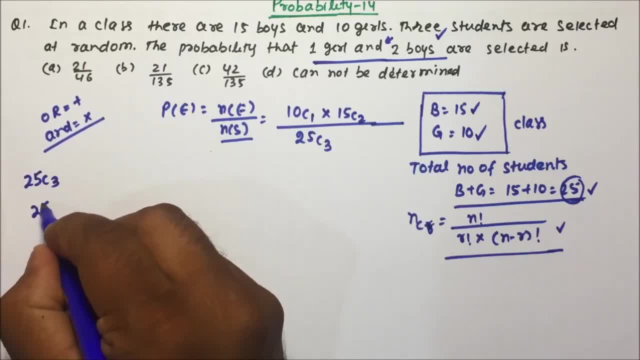 calculate 25 C 3.. So 25 C 3 will be 25 factorial divided by 3 factorial, N factorial, R factorial into N minus R factorial. So 25 factorial will expand 25 into 24, into 23, into 22 factorial. We will stop. The reason is: if you have 2 boys and 2 girls, you will be able to add those 4 boys. So the probability that you will have 2 girls is 25 C 3 divided by 25. factorial. divided by 3 factorial. 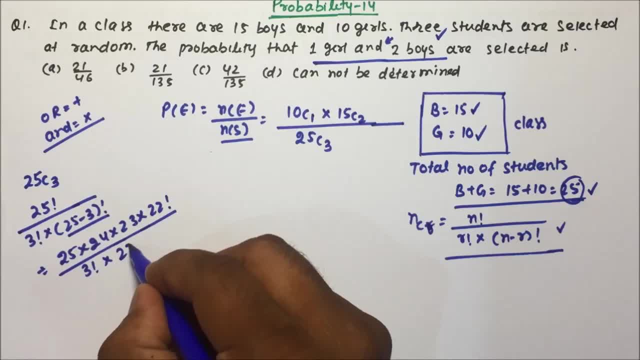 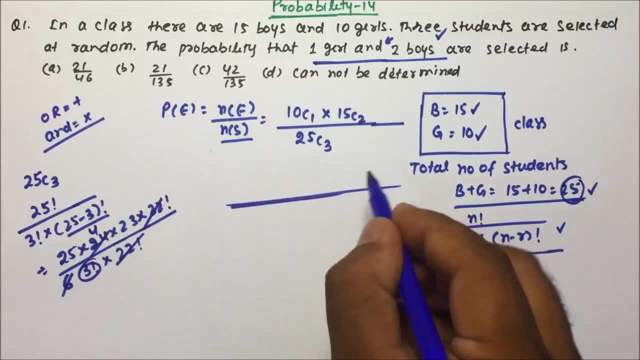 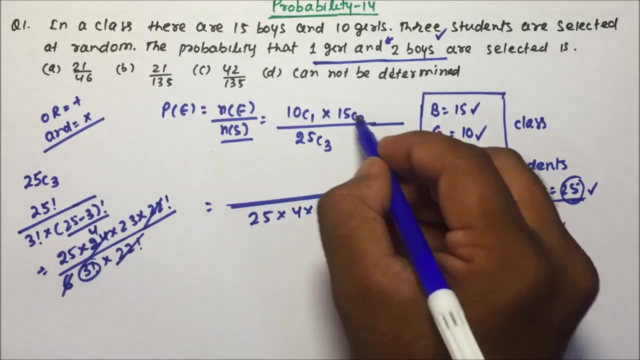 in the denominator also, we have 22 factorial, so the gone 3 factorial will be nothing but 6, so 6 forja, so i can write the denominator will be. so i can write the denominator will be 25, into 4, into 23. i will not multiply it here. then, friends, 10 c 1, 10 c 1 will be 10 and 15 c 2. so 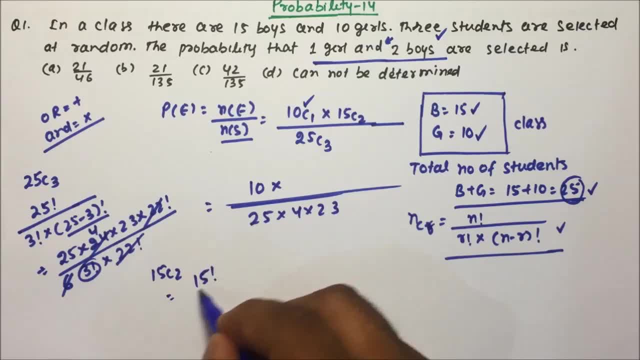 15 c 2, if you calculate, then it will be 15 factorial divided by 2 factorial into 15 minus 2 factorial. so 15 factorial divided by 2 factorial is 2 and 15 minus 2 will be 13 factorial. now if 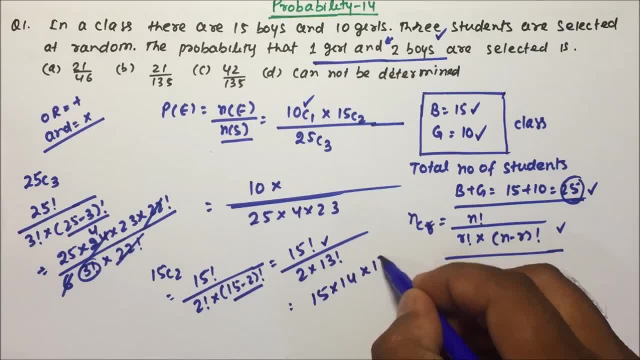 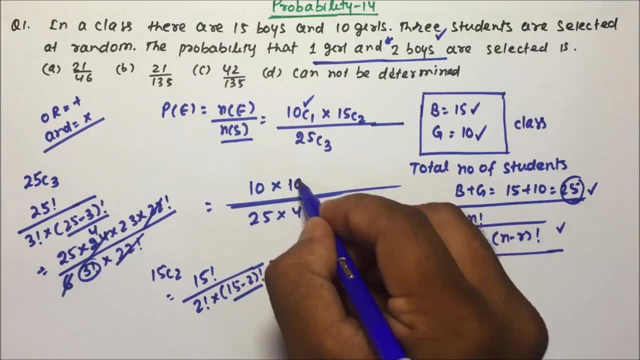 you expand it then 15 into 14 into stop till 13 factorial and 2 into 13 factorial. here this is gone to 7 times. so 15 into 7 will be 105. now, friends, you can see a 5, 5ja and 5, 2ja and 2. 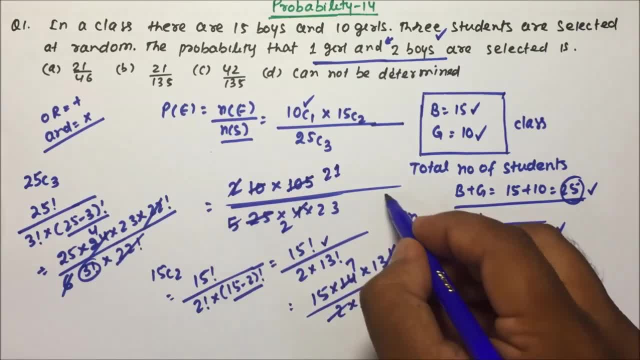 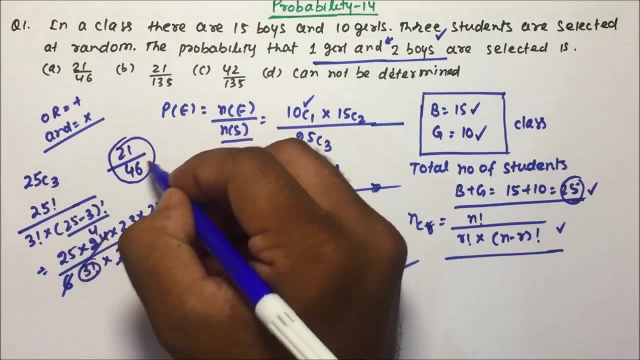 21 times, and this is 2 will cancel this 121 times, and this is 2 will cancel this by 2 times, So 21,. so 21 divided by 2 into 23 will be 46.. So 21 divided by 46 will be the answer. 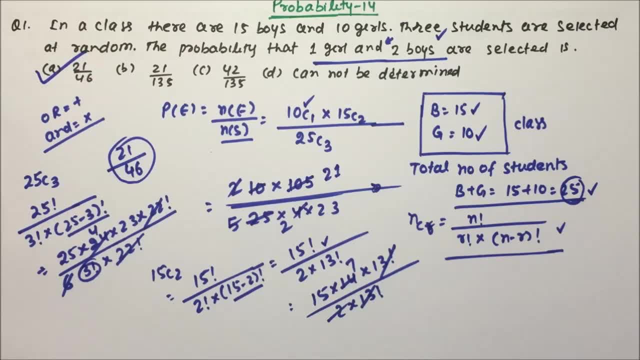 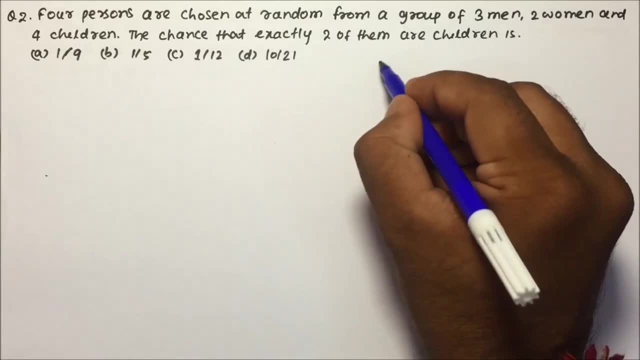 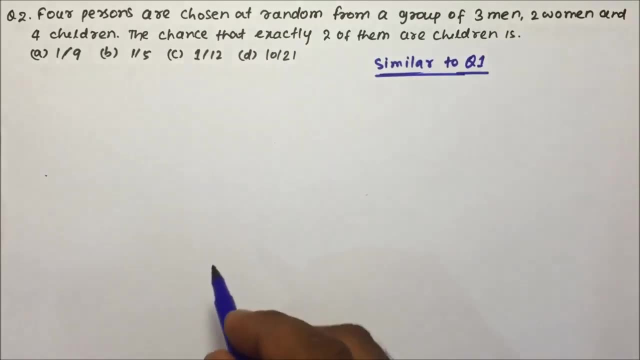 So option A will become the correct answer for question number 1 and this kind of question you can expect in your exam, friends. Now moving towards the question number 2.. Now, question number 2 is similar to question number 1.. So let us see how we are going to solve this. 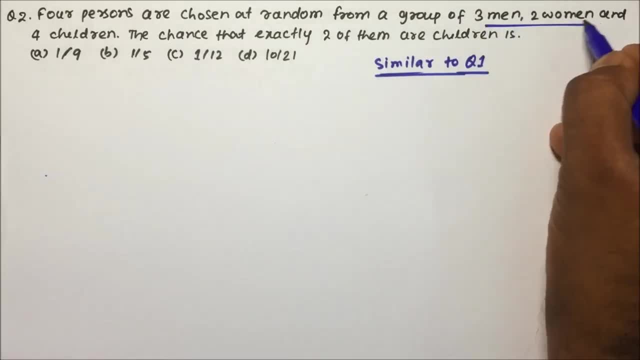 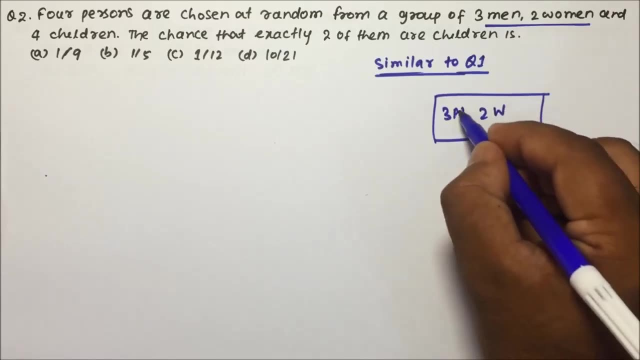 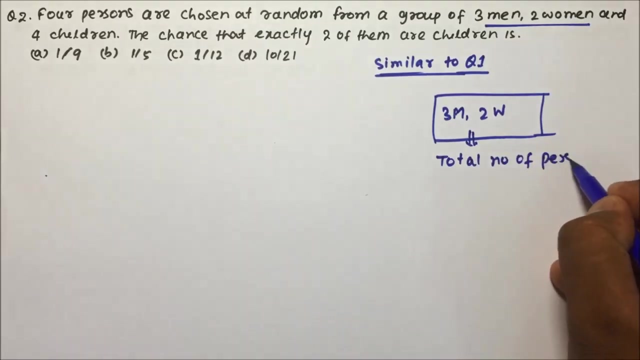 Four persons are chosen at random from a group of 3 men and 2 women. So there is a group, is there of 3 men and 2 women? So, friends, total number of total number of person. So total number of person: if you will calculate, then it will be 3 plus 2, which is nothing but 5.. So total number of person. 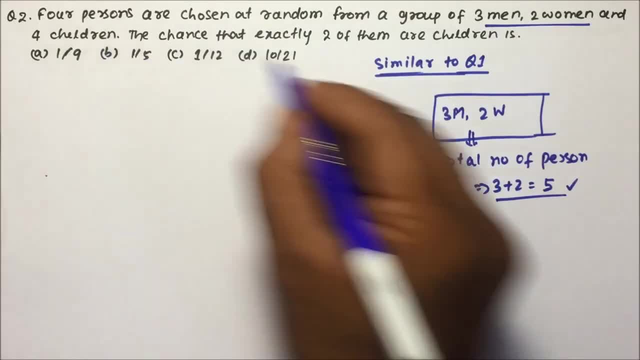 we have got here is 5, and 4 children are also there, So 4 children. So total number of person will be 3 plus 2, which is nothing but 5.. So total number of person we have got here is 5.. 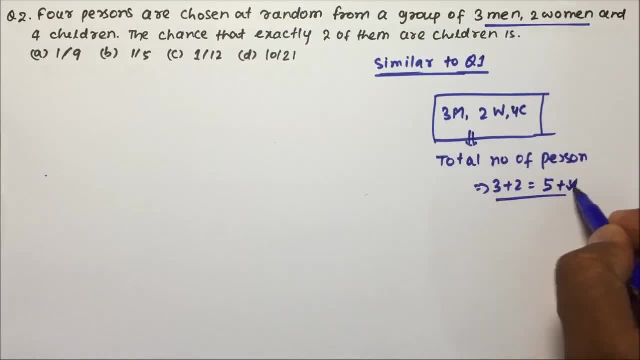 be 3 plus 2. 5 plus 4 is 9. so again we will add 4 plus this. so total number of person will be 9. so this total number of person is having 3 men, 2 women and 4 children. now the chance is that. 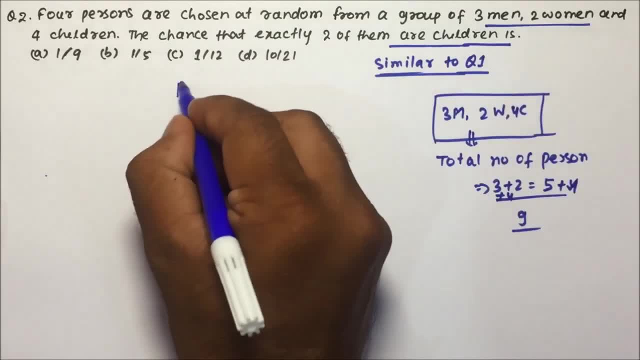 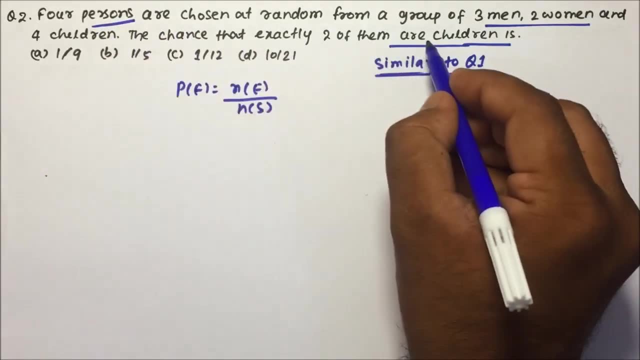 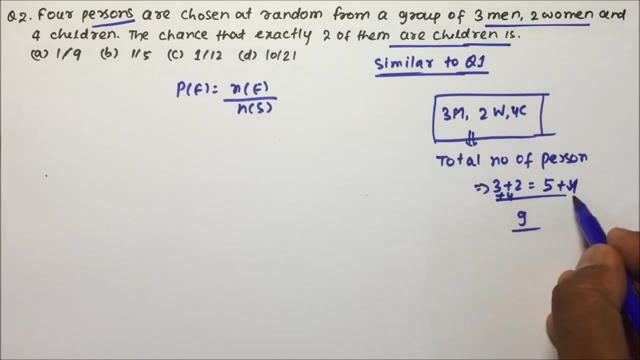 exactly 4 of them are children is now friends, my probability will be equal to ne divided by ns. right, okay, so total number of person: so 4 persons are chosen at random from a group of 3 men, 2 women and 4 children. so total number of person is nothing but 3 plus 2, 5, 5 plus 4 is 9, so total. 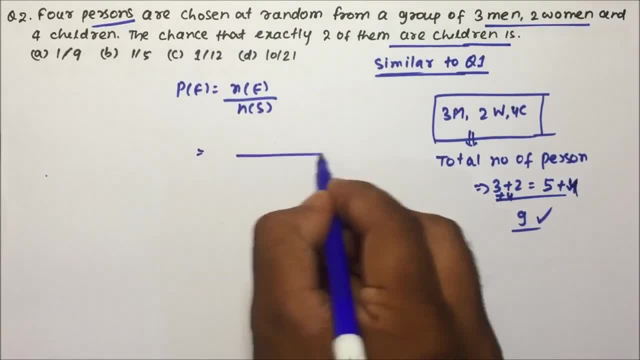 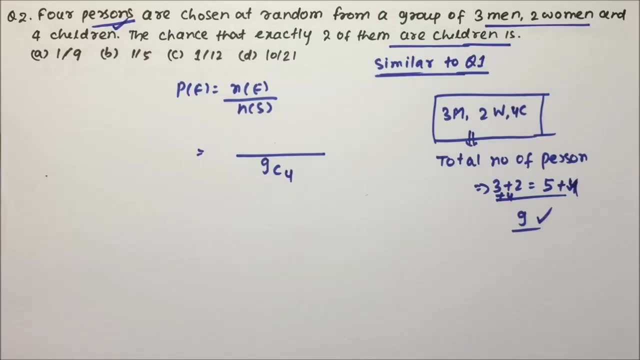 number of person we have is 9. so how many persons are chosen at random? so out of 9 we are choosing 4 persons, so 9c4. so this will become my ns. total outcomes now favorable outcomes. so you want exactly 2 of them are children. so if you want exactly 2 of them are children, then 2 you select. 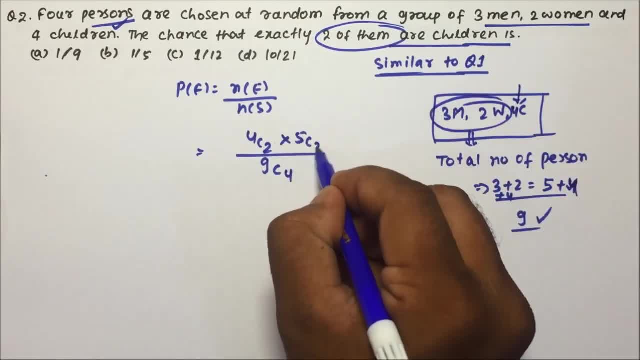 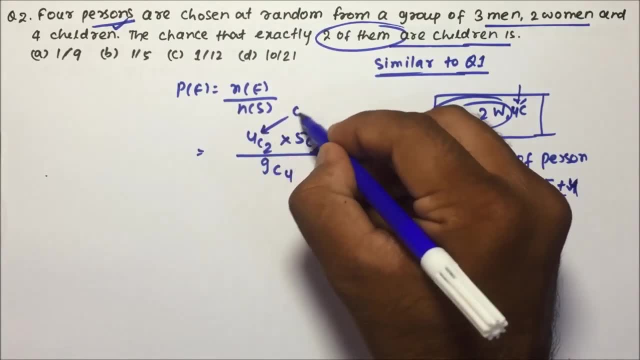 from the children and the remaining 2. the remaining 2 you select from the children, the remaining 2 you select from the main and domain. See, there is a condition friends try to understand. So there is a condition only on the children. They want exactly 2 children. 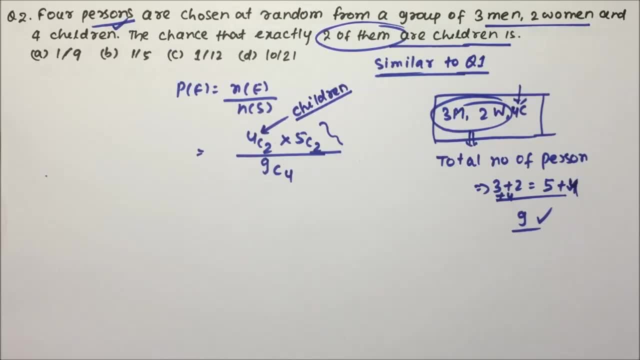 and they are not worried about main and domain. So that will become 5c2.. Now, friends, 4c2 into 5c2 and divide by 9c4 will give you the answer. So 4c2, 4 factorial, divide by 2 factorial into: 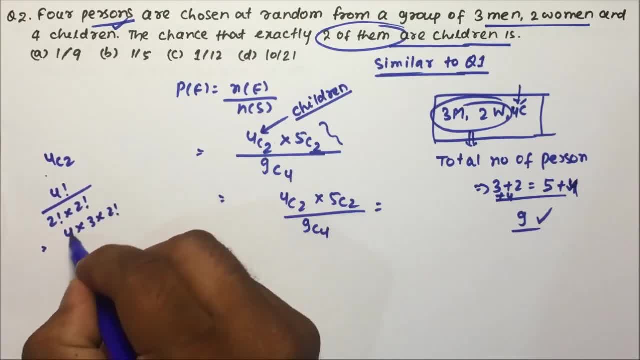 2 factorial. So 4 into 3 into 2 factorial, or 4 factorial is 24.. 2 into 2 is 4.. So this will be getting 6.. 5c2 if you calculate 5c2.. So 5 factorial divided by 2 factorial into. 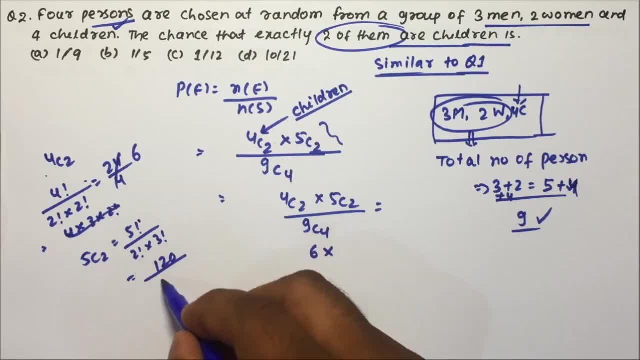 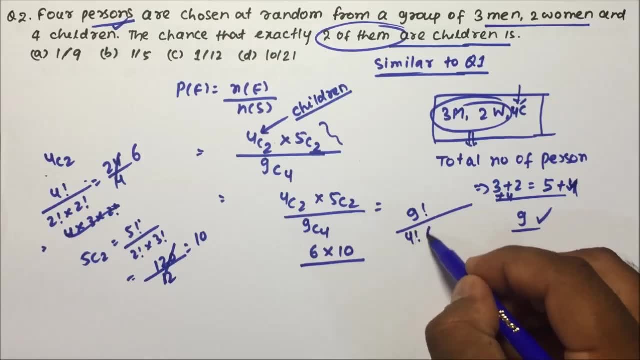 3 factorial, 5 factorial will be 120.. 3 factorial is 6.. 6 into 2 is 12.. So this will be getting 10 divided by 9c4.. So 9c4 means 9 factorial divided by 4 factorial into 5 factorial. So 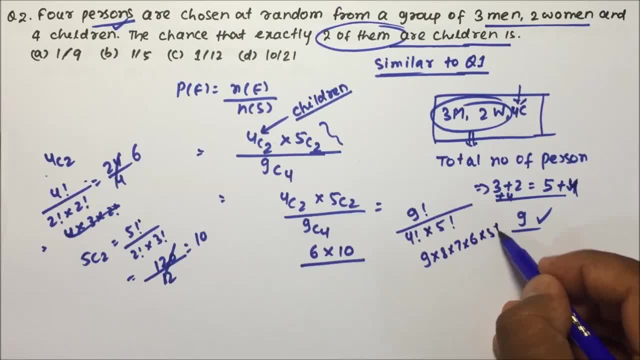 9 into 8 into 7.. 9 into 6 into 5 factorial. divided by 4 factorial will be 4 into 3 into 2 and 5 factorial will keep it like this: 5 factorial, 5 factorial cancel and 4: 2ja will be 8 and 3 into 2.. So